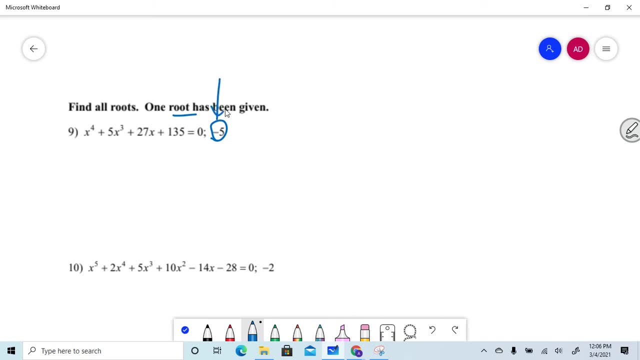 is a root, all right. So hey, FYI, since negative five is a root, then you know that x plus five was a factor. by the way, Just take a note of that. It's probably going to be helpful in the. 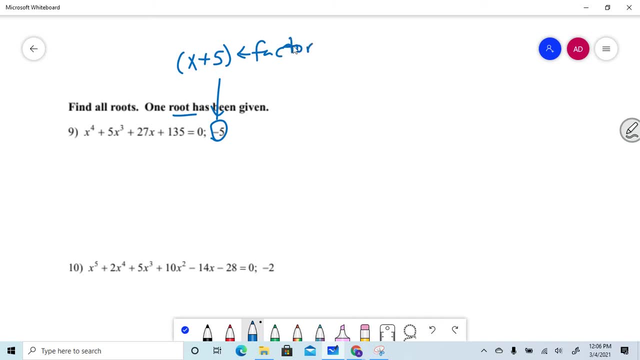 later video. okay, So you know x plus five was a factor, Okay. so if you're given the root, take the root, put it in the little corner, okay, And basically line up your coefficients. I have a one, a five. Remember what we said. if you're missing a term, put the zero, okay. 27 and 135.. 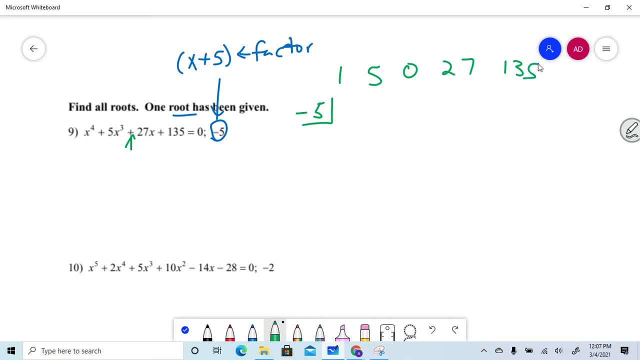 So what am I doing? I'm using all right, maybe not using very well. I'm using synthetic substitution slash division to help me solve a polynomial equation. I know so much going on, I can't even stand it. Okay, here we go. We drop the coefficient right, Drop the leader. Multiply gives me negative five. 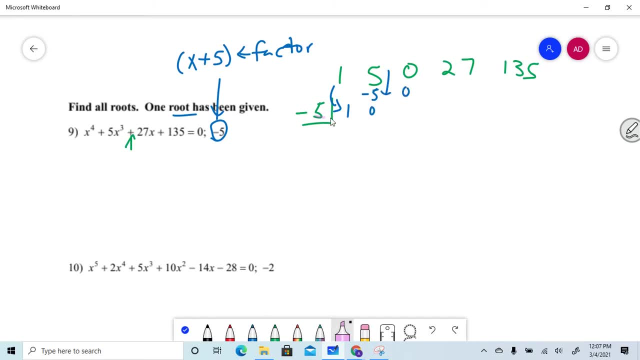 We drop it, We run it. Remember what I said in my other videos? right, You're multiplying up to get that? okay, Then we drop it. all right, We run it, We drop it, We run it And lo and behold. 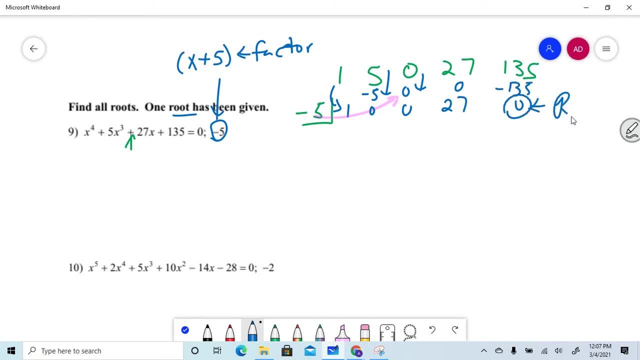 wait for it, wait for it. Yep, the remainder is zero. Of course, the remainder is zero. We know the remainder was zero because, oh, by the way, we were told, this was a root, It came from a factor. 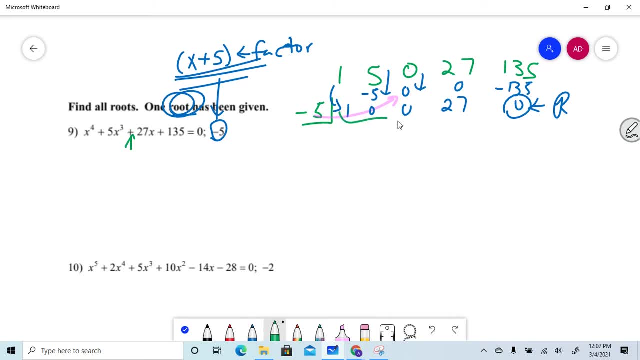 right, Okay, we got that. Now these numbers right here represent the coefficients of the depressed equation. So in other words, that's an x cubed plus zero, x squared plus zero x. we don't need that right, But plus 27.. Now remember what I said: this is my depressed 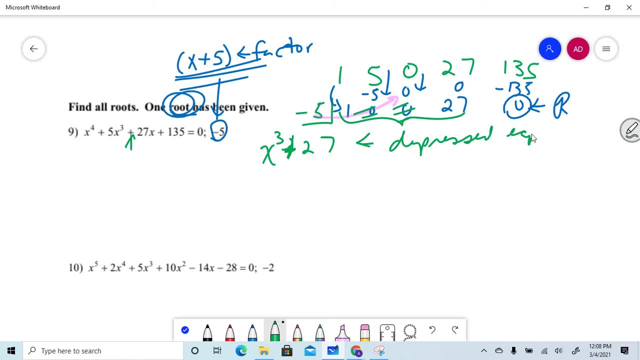 equation, meaning I can solve this because- oh, by the way, it's a cube term, So I set it equal. Now you're going to have to remember that you have to be able to factor a cubed plus b cubed. 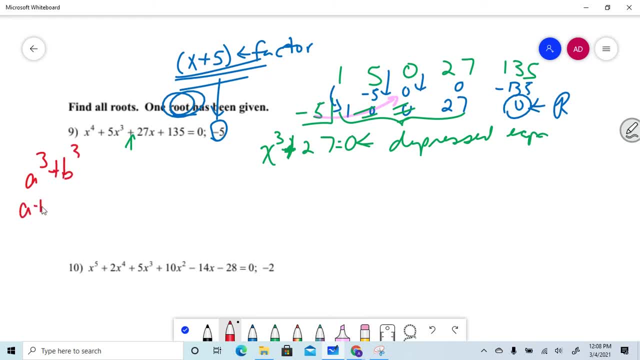 okay. So that's one of those things way back when It was another video. I'm just saying you might want to go check it out. And I get a plus b, a squared, minus ab plus b squared. okay, That's how you would factor that. So to factor this, my a is x, My b is three. 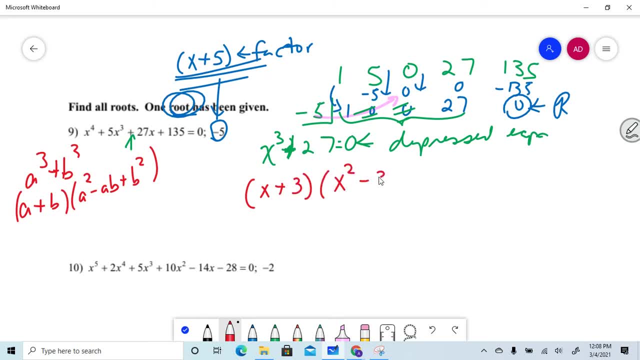 So I go x plus three, x squared minus three, x plus nine, because that's b squared right And it equals zero. Now check it out. I have another factor. I could set that equal to zero and solve. So guess what? 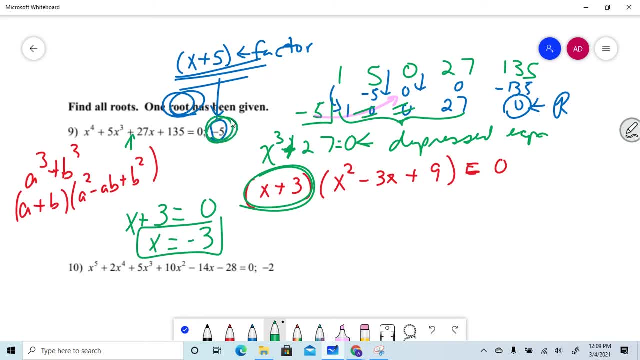 I found another root. So not only was five a root, negative five a root. x equals negative, three is also a root. So now all that's left is to solve this equation. Oh, but wait, guess what? That's a quadratic equation, And way back when a galaxy not so far away. 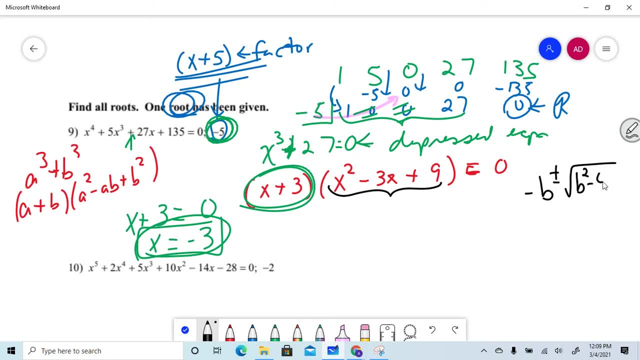 You watched a very cool video on the quadratic equation: how to solve a quadratic equation using, I know, the quadratic formula. Super, super exciting. So here we go. Negative b plus or minus the square root of b squared minus four times a, times c over two a, And it really 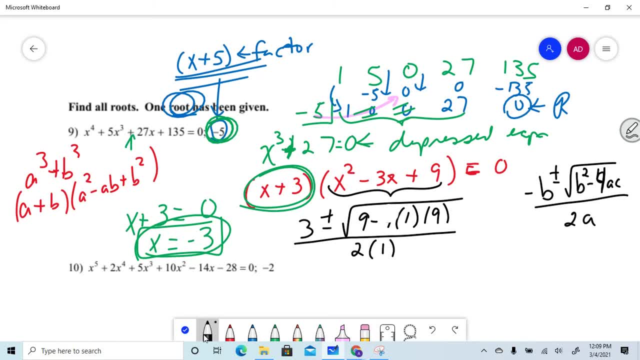 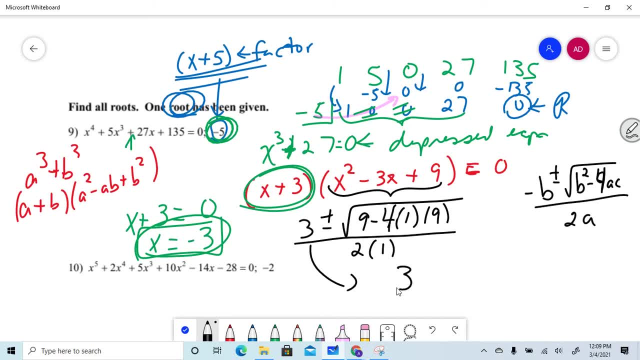 swear, I swear, I swear. Okay, So here we are again. three plus or minus the square root of nine minus 36 over two, which, of course, is three plus or minus the square root of negative 27 over two. And feel free to pause the video if you have to. I'm totally okay with that because you know what. 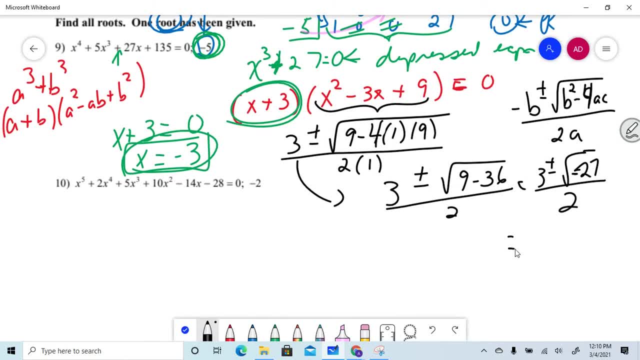 I wouldn't even know if you did Okay. So now when I kick all this out, I get three plus or minus three. i square root It's a three over two. And you might be like, what the heck? Where did that i come from? 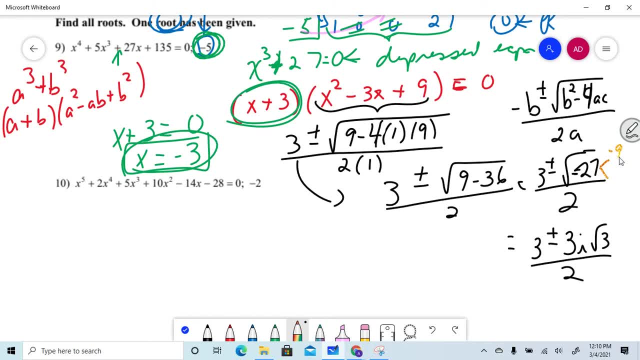 Well, you might want to watch another video, or you can just say, oh wait, that was negative nine times three. And then, of course, the square root of negative nine is three. i and the radical three is just saying inside of the house: Okay, So look at all these roots we have. Okay. So my final. 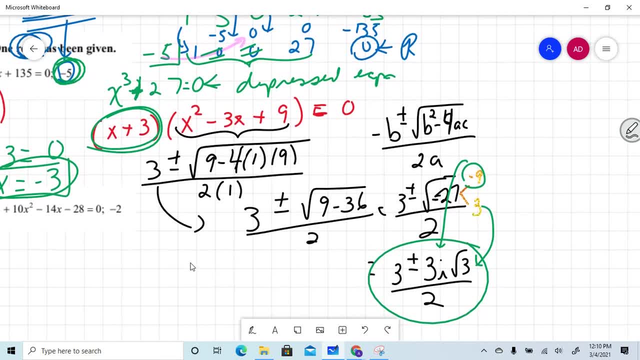 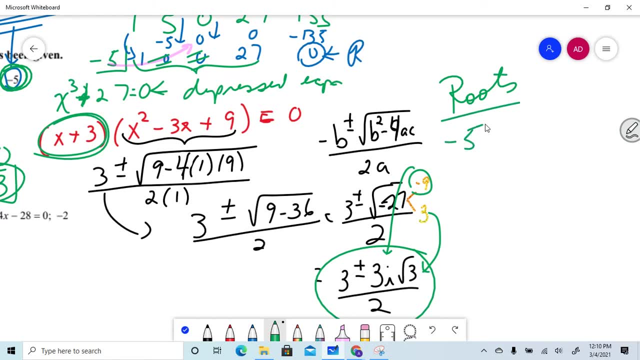 answer has a few of these roots. Okay, Not a few, It has all of them. Okay, I have my roots are. I'm going to write them over here just to make it all nice and neat, crazy, fun. negative five is a root, Negative three is a root, And then, yeah, those guys are also a root. 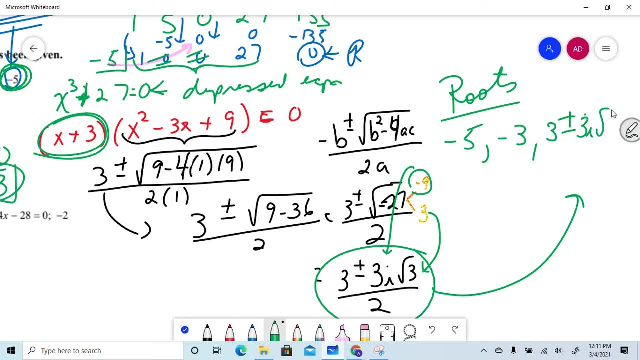 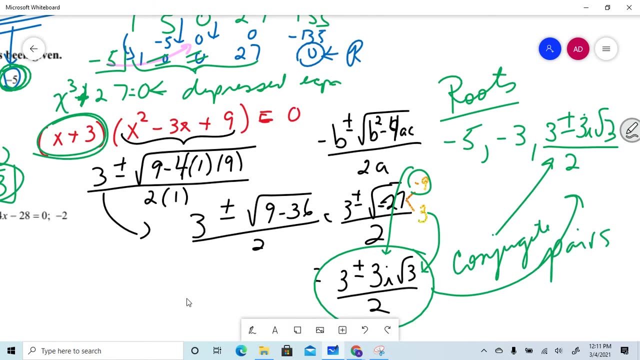 So remember, there are two roots here. I think sometimes we forget that there's actually two roots because it is a conjugate pair, right? Remember we talked about that in class, right? Imaginary roots always come in conjugate pairs. Super, super exciting, I know. All right, Okay. 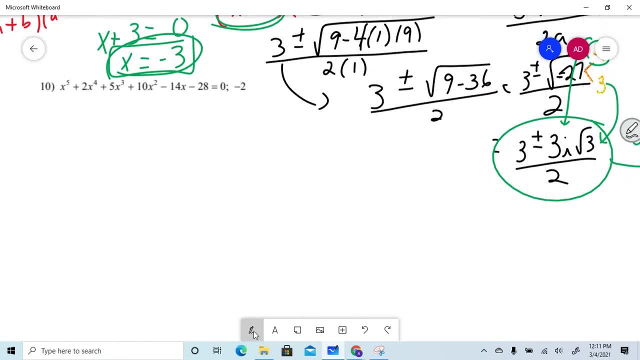 Feel free to pause the video. Do what you got to do, right, Because guess what? We're moving on to the next one. I know, Super, super Okay. Now I'm going to try to go a little faster, So you might want to hold onto your seat. Here we 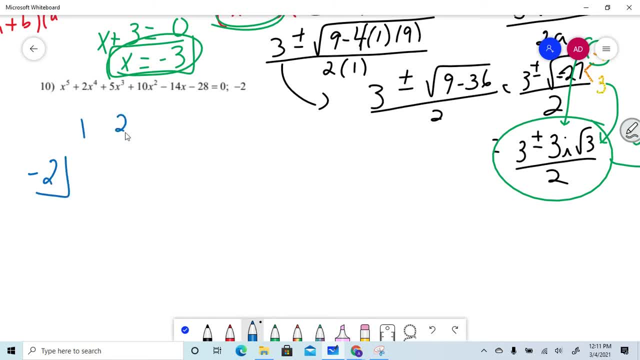 go, Take your root, put it in a little corner. line up those coefficients: One, two, five, 10, negative 14, negative 28.. Okay, Just please note. if you were missing a term you would have had to. 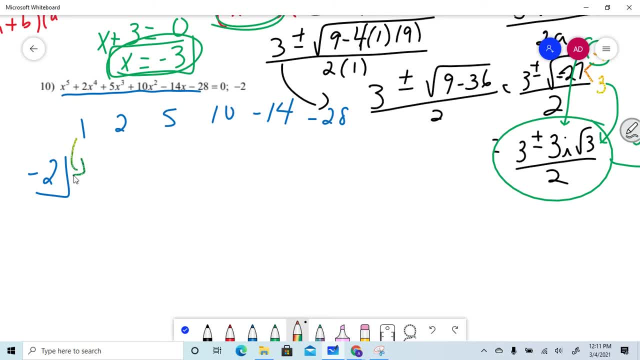 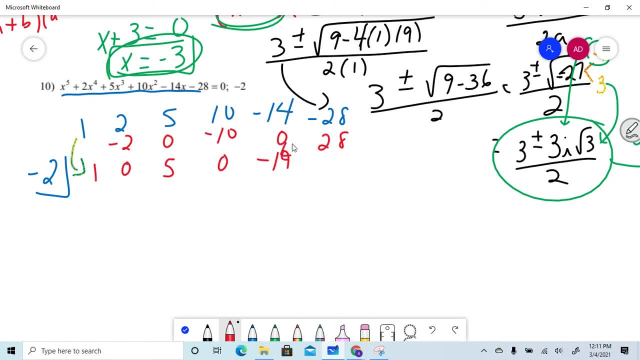 drop it, run it. That's a 14.. Oh my God, I can't understand it. That's zero. We knew it was going to be a zero remainder, because negative two was a root. How many times do you need to hear me? 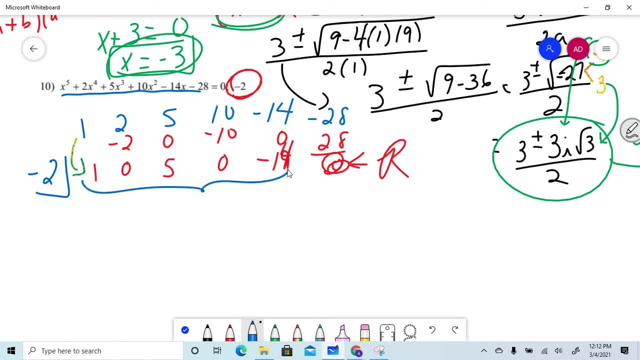 say that I know Crazy fun. All right. So now look at what we got over here. Since I started with a degree of five, this is going to be a degree of four. Then I have a zero X cubed. Well, 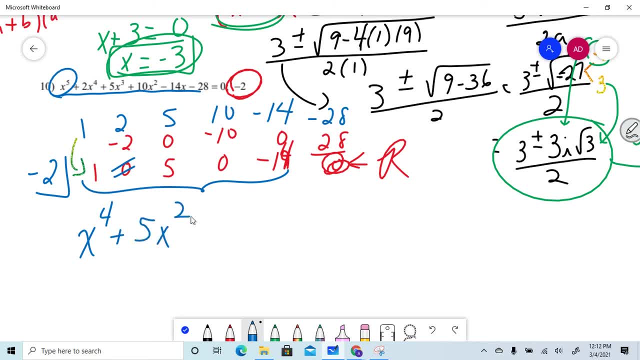 I don't need to write that, but I do have a five X squared. Then I have a zero X. Yeah, you don't need to write the ox. Ha ha, ha ha, I know right, Funny. And then I have a constant, So I put negative 14.. This is my depressed. 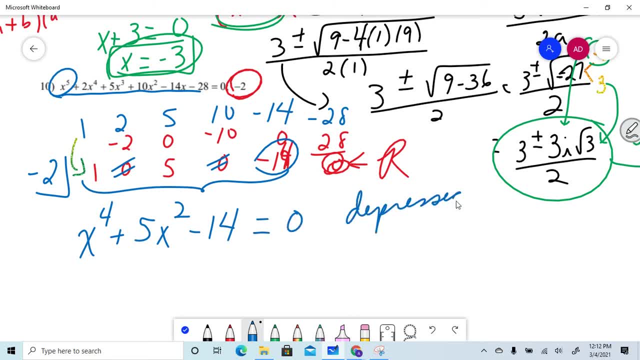 equation. Not because it's sad. Please don't think it's depressed because it's sad. It's actually kind of happy because we can solve this. I know Super, super fun. So this gives me X squared plus. sorry about that, X squared plus seven and X squared minus two. So you might be. 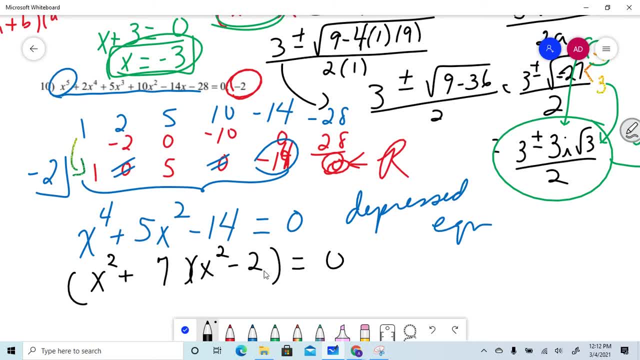 wondering: well, wait a minute, How did she get seven and two? Okay, So remember, I'm looking for factors of 14, of negative 14 at that, that are going to combine to get me a five, a positive five. So that's why it was a plus seven and a minus two. Okay, So this: